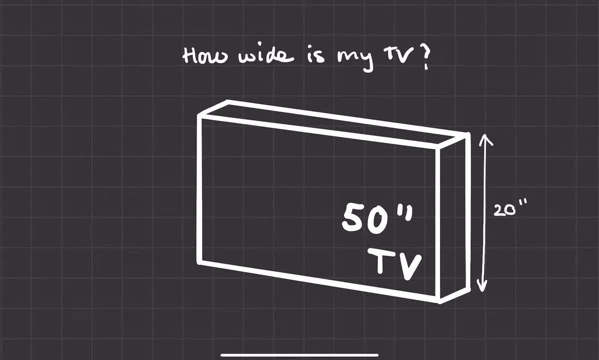 TV in a box, And you might know that TVs when you measure them. so if you say I've got a 50 inch TV, then that means the diagonal length of the TV is 50 inches. So here I've actually got a right-angle triangle. I've got the height of the TV. I've got 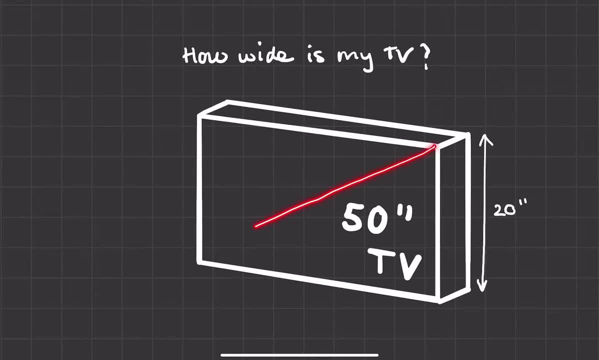 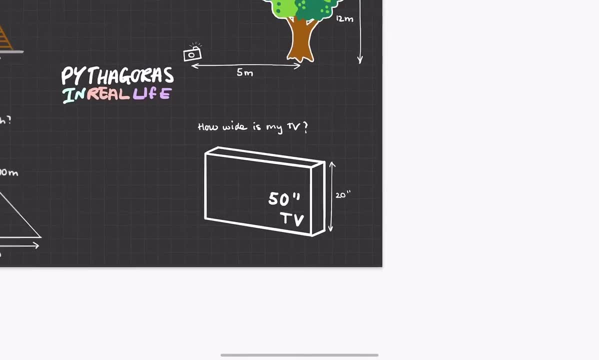 the width of the TV and I've got that diagonal length there, So this makes a triangle here, a right-angle triangle. Okay, this one's just in 3D, So we can work out missing lengths using Pythagoras. So why don't you pause the video? see if. 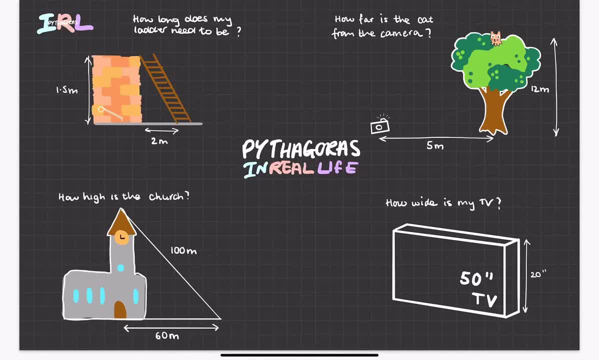 you can work out what they are for each one of these, and then I'll show you the answer. Okay, so let's have a look at the first one. So here I've got some length of the ladder. let's call it X, and we know from our Pythagoras that 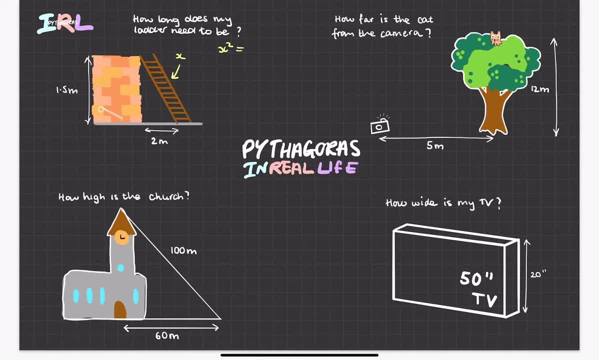 the hypotenuse squared is equal to the sum of the squares of the two shorter sides, And so if I want to know what that distance is there, how high my ladder is, I can do the square root of all this, and that gives me an answer of 2.5 meters. 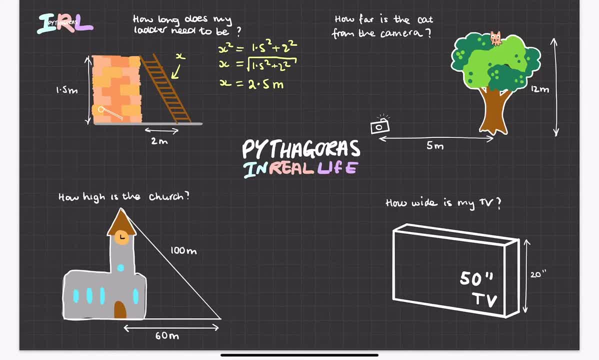 You might have to do that on your calculator For this cat over here. so this is the triangle I've got, Okay. so I want to know how far away the camera is from the cat. And again, let's call it X, and that's the hypotenuse again, isn't it? So the 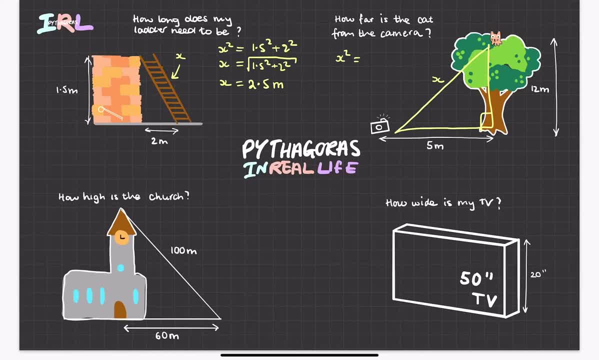 hypotenuse squared is equal to the sum of the squares of the two of the sides. So if I want to know what X is, I have to do the square root of all that And that gives me an answer of- let's do it on my calculator: 5 squared plus 12 squared, that gives square root of it. that gives me 13.. 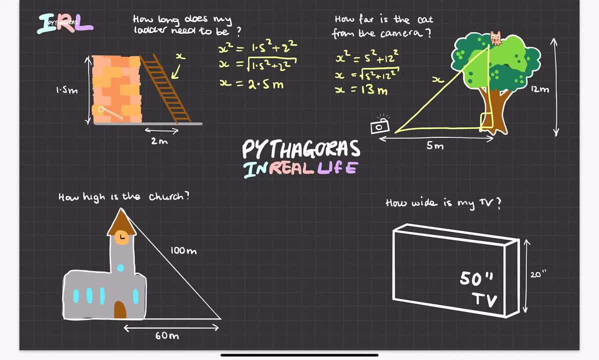 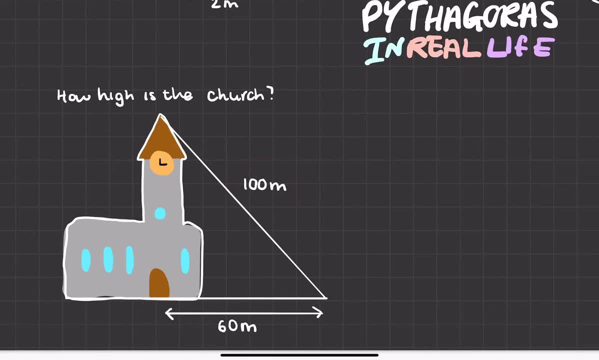 Meters, Okay for my. how high is the church? Okay, for some reason, I know this, don't know how I know this, but I do, And we can make a triangle here. So this time what I want is one of the shorter sides, So let's call it X again, But this time. 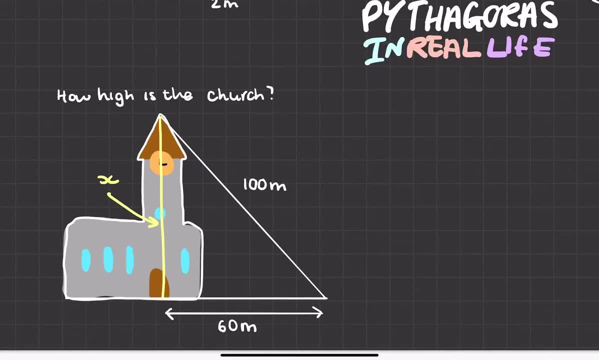 because this is the hypotenuse, I'm going to write out my Pythagoras' Theorem: the hypotenuse squared is equal to the square root of all the squares of the two of the sides. So this time, because this is the hypotenuse, I'm going to write out my Pythagoras' Theorem: the hypotenuse squared is equal to the square root of all the squares of the sides. 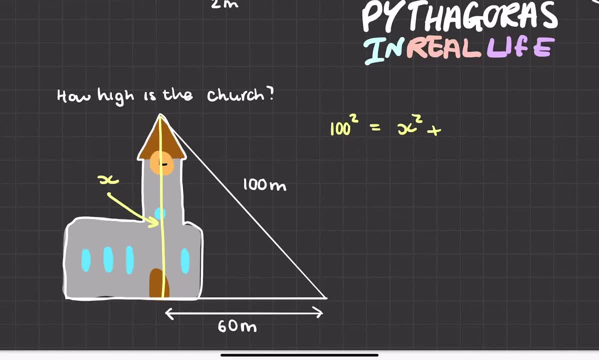 So this time, because this is the hypotenuse- squared is equal to the square root of all the squares of the sides. Okay, so you think about your factor: families, X squared must be a hundred squared. take away 60 squared and we're going to square root all that, So a hundred. 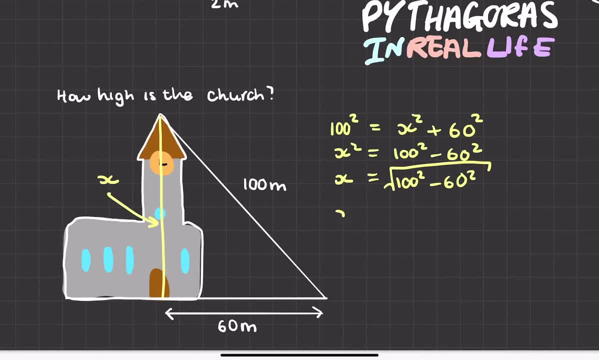 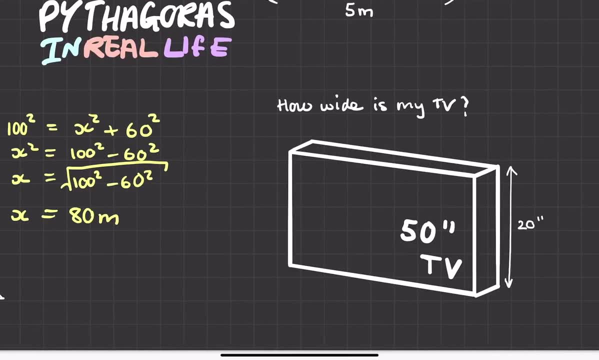 squared. take away 60 squared and that gives me an answer of 80 meters. And then the last one. here I've got: how wide is my TV TV? so here this is kind of in 3d this. it's like a three-dimensional picture. so 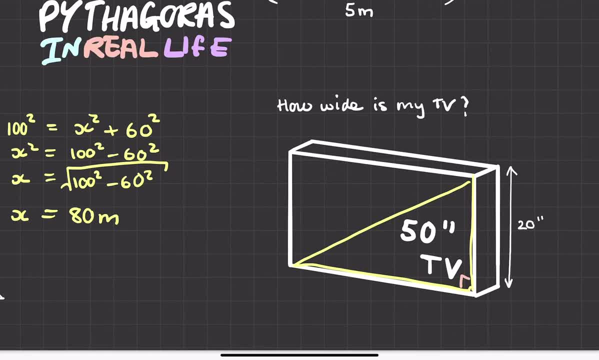 this is my right angle down here. I know that it's 20 high. let's make that 20. that's 20 high and I know the diagonal. that length there is 50. this is in inches and let's say I want to know how wide it is. let's call it X and we'll 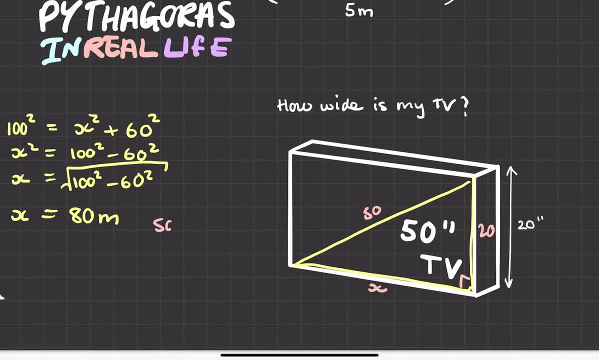 write down the Pythagoras theorem. so we'll write down: 50 squared- because that's my hypotenuse- is equal to x squared plus 20 squared. think about your fact: families. so x squared equals 50 squared. take away 20 squared and then we're going to square root that. so on my calculator that's gonna be the square. 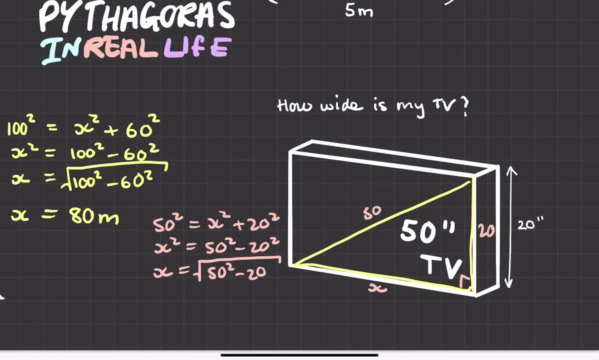 root of 50 squared minus 20 squared. let me type that and see what we get: 50 squared, take away 20 squared, that gives me an answer of forty five point eight, three inches. so here I've rounded up two decimal places, okay, and so that's a. 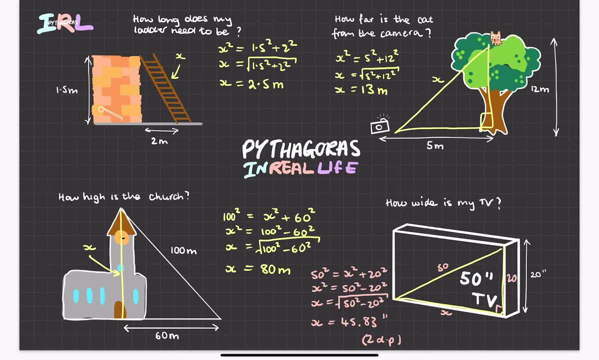 quick look at how we might recognize Pythagoras and that when to use Pythagoras in a real life situation.